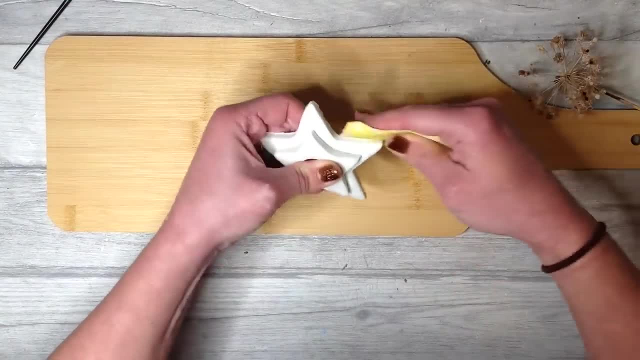 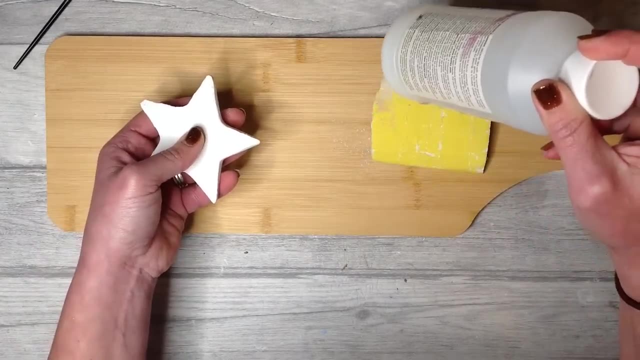 The air dry clay is now fully dry and I have a small piece of sandpaper and can smooth down any imperfections and edges. Make sure you seal the clay and then it's ready to use. Really simple, but really effective. I love how this has turned out and this will look. 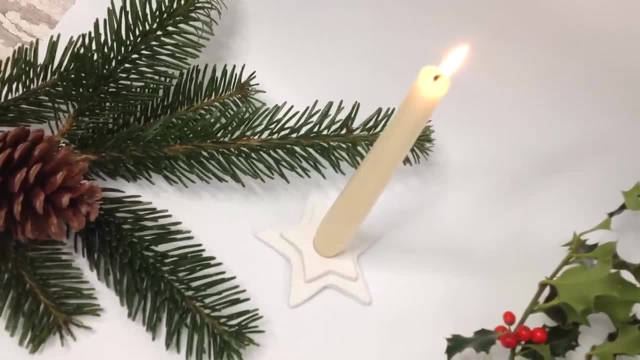 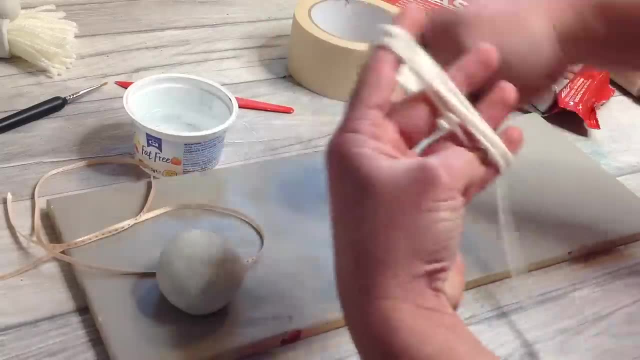 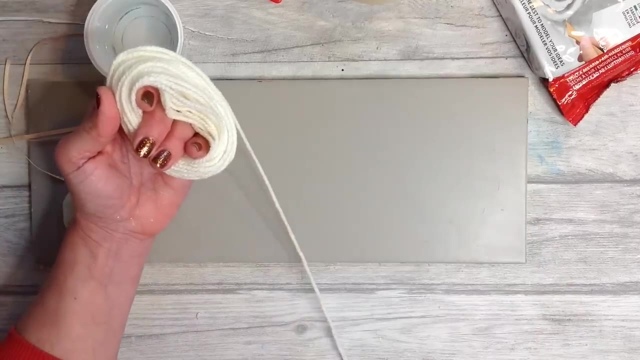 lovely on my Christmas table. This next project is a really fun Christmas craft and we're going to make a gonk decoration. Take some wool, yarn or string and make a large tassel. I'm making my ball of wool really quite fat and plump around my hand like this. 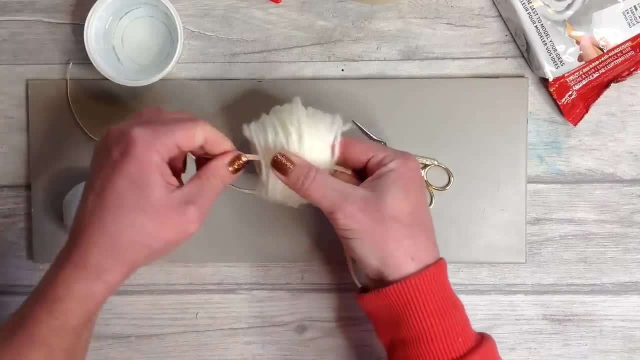 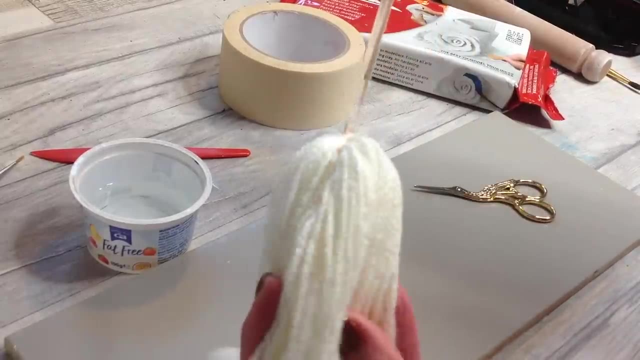 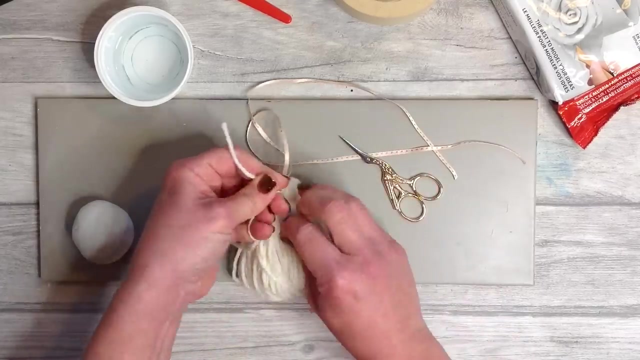 Take a long piece of ribbon and tie it in, like I do here, nice and securely. Make sure the ribbon is nice and long, as you can see- and we're going to be using some air dry clay for this project as well- I'm tying the tassel together with another piece of yarn, then snip the loops on the. 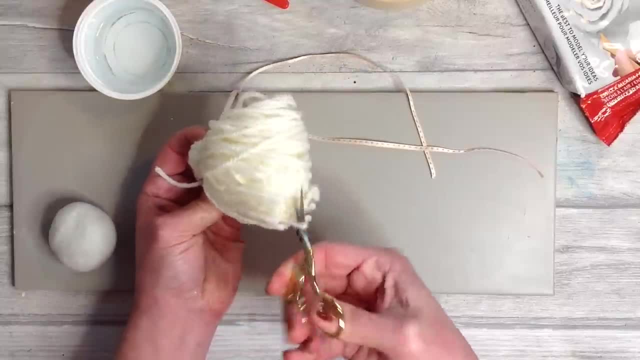 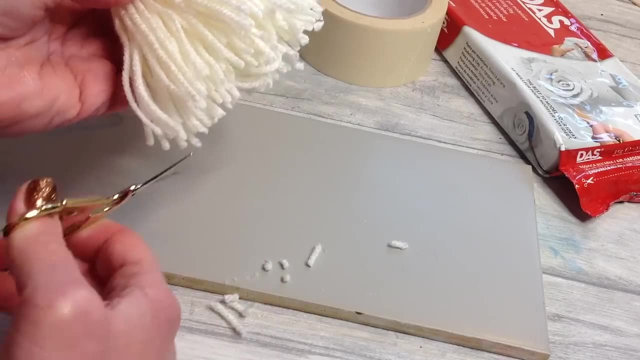 longest end, then using the scissors to tidy it up and make the ends all nice and neat. There are so many uses for this kind of tassel, but this is by far the cutest one I've ever come up with and hopefully quite an easy Christmas project for you to do as well. 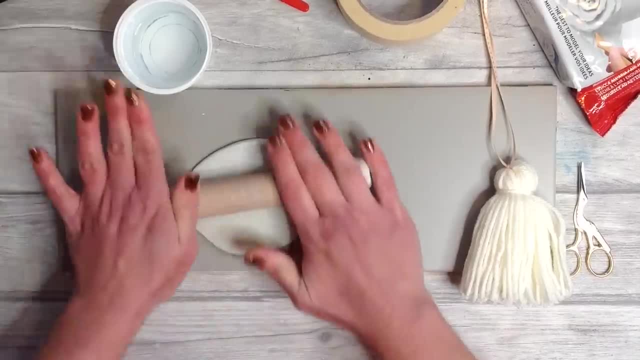 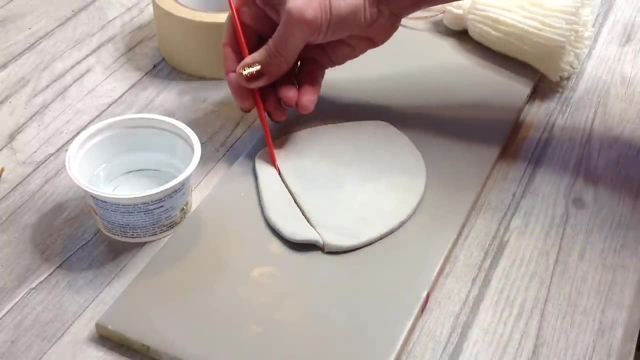 I'm rolling my ball of air dry clay out, like I did before. I've rolled it with a nice curved edge like this. but if you don't have a curved edge you can cut it. and then we want to cut a rough kind of triangle shape with rounded edges. 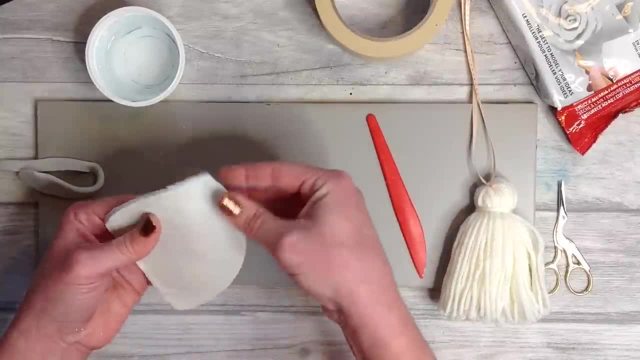 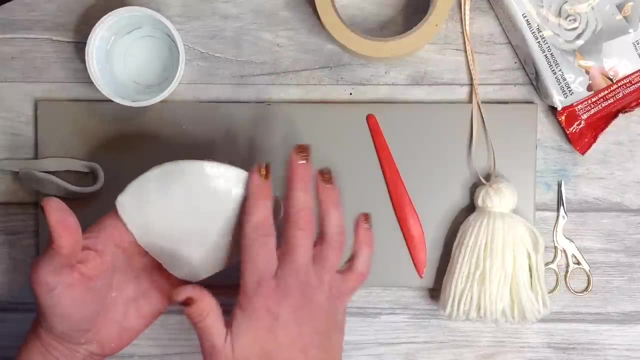 This is perfect, as air dry clay is very forgiving and very mouldable. I'm just tidying up the edges a little bit and this is going to be the gonk or the gnomes little hat. To get the size correct, I now bring in my yarn tassel and wrap this around just at the 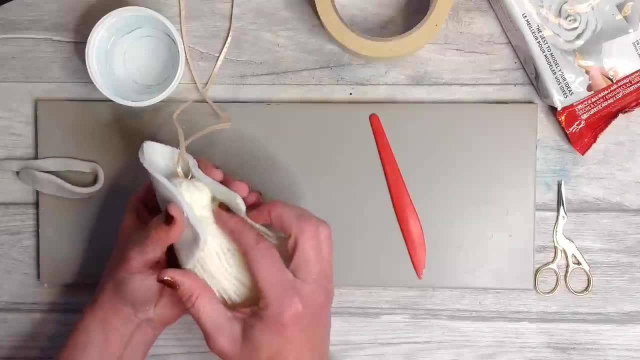 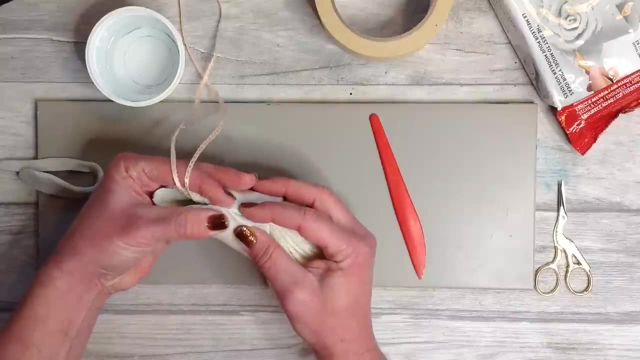 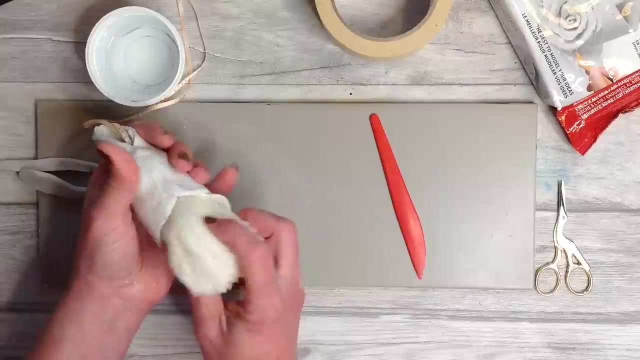 top, Tuck everything in nice and neatly- and please note, I've just been and washed my hands so I'm not getting all that air dry clay all over the wool or the yarn- Pinch and join the hat together like you see here. To finish off moulding the hat, I like to take the tassel out. 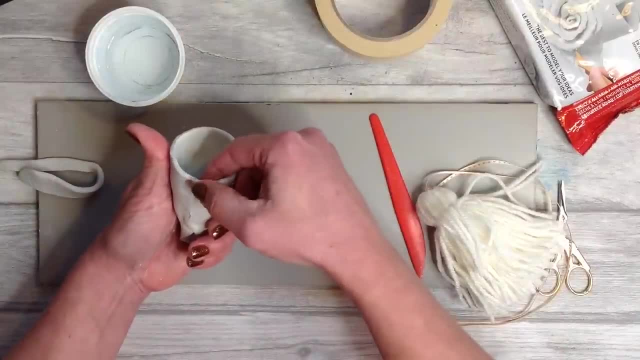 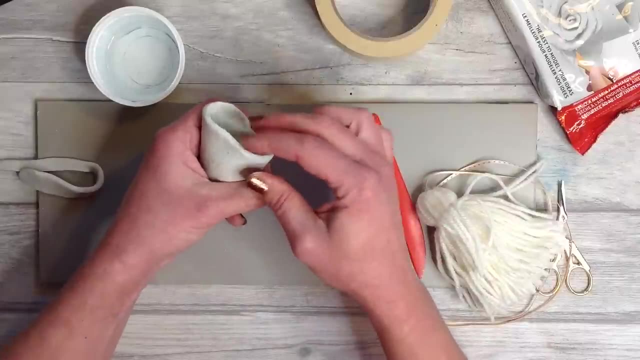 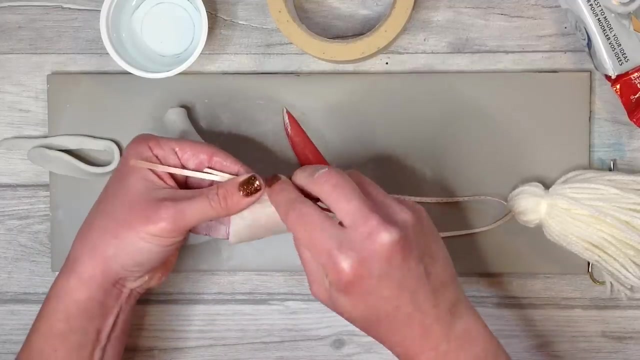 This just gives us a little bit more freedom to mould and to blend and to really get those edges lovely and smooth. but don't forget to leave the very tip of the hat open, as we need to put the ribbon back through there. And to do this I wrap the end of the ribbon in a little bit of tape so that I can easily 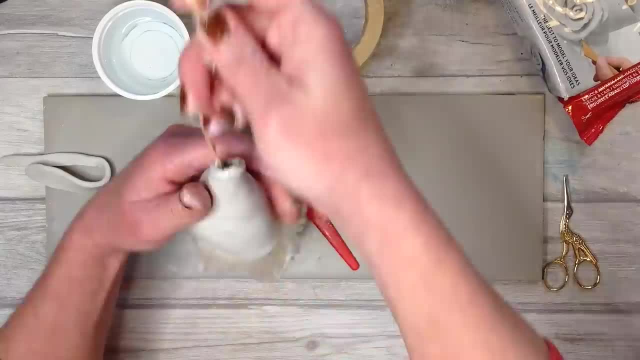 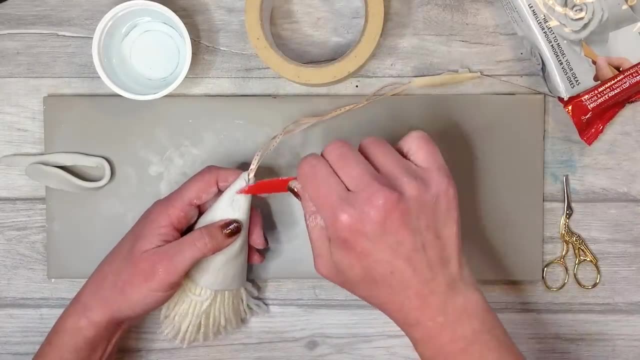 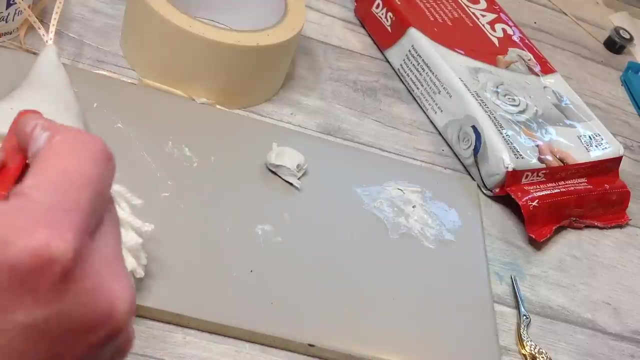 push this back through the hat, Close up the gap in the air dry clay and make it lovely and neat. Don't worry if this process all takes you a little bit longer. it just takes quite a bit of practice For the nose. I've rolled a ball of air dry clay and I'm going to use the score and slip. 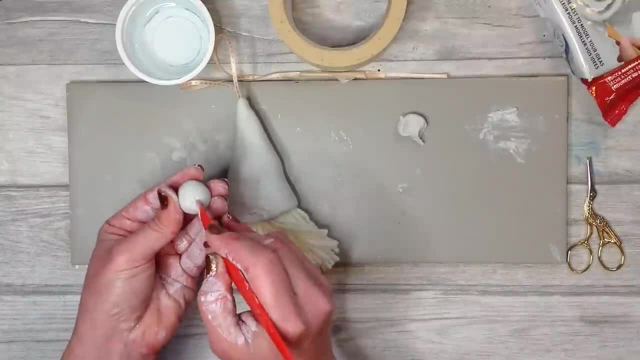 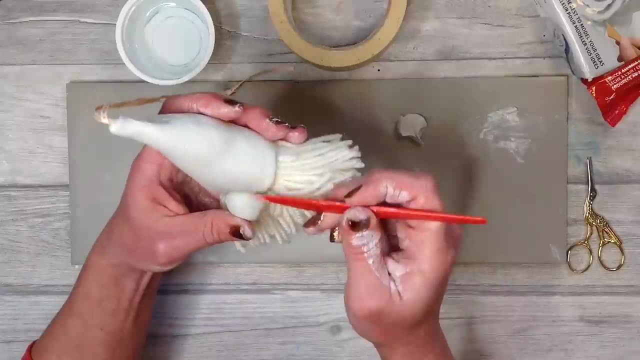 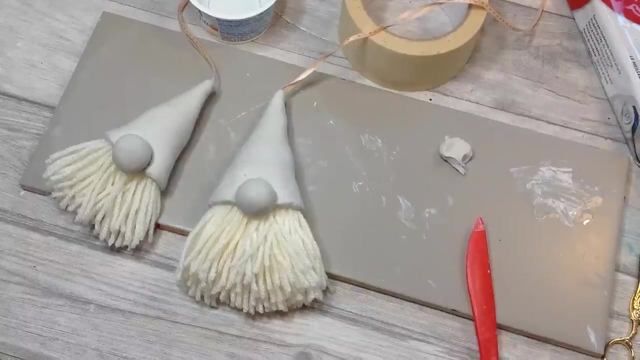 method once again to attach this in place. As you can see, our little gonk decoration is starting to come to life. now, Once that's adding on there, Make sure you knit both sides together by pushing one side into the other. If you like them like this, then you can leave them to dry at this stage, but I wanted to. 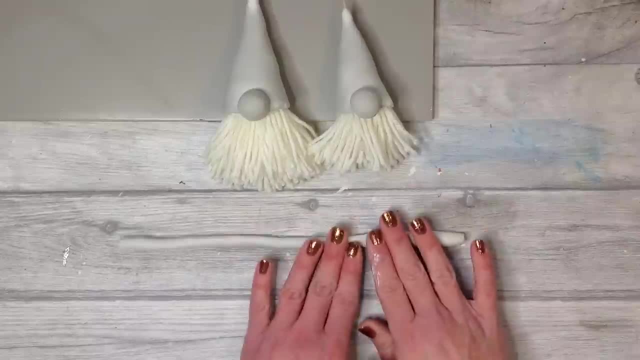 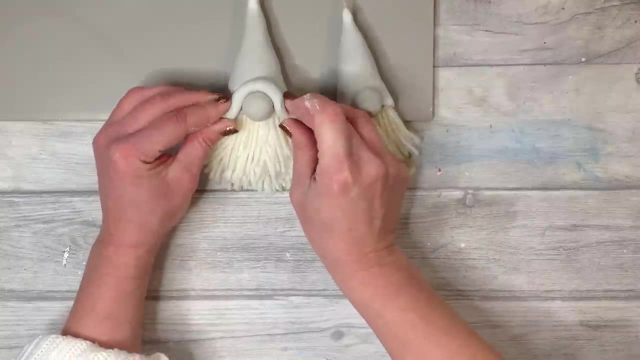 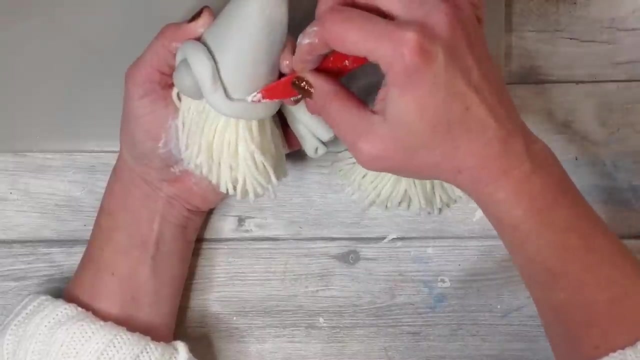 add a little extra detail and I roll a nice coil and I'm going to add this around the bottom section of the hat so it really makes it look like that nose is popping out from underneath the hat. Using the score and slip method And 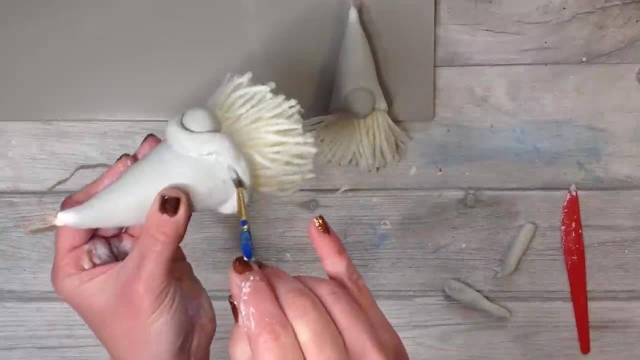 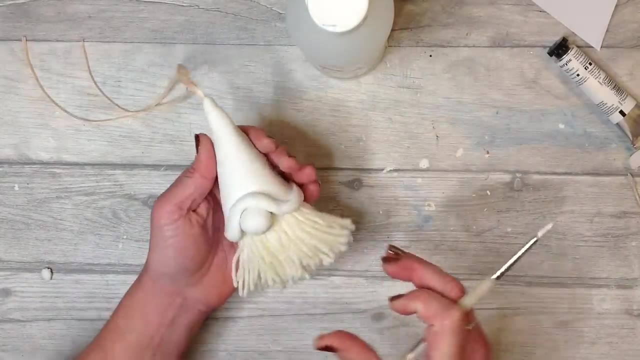 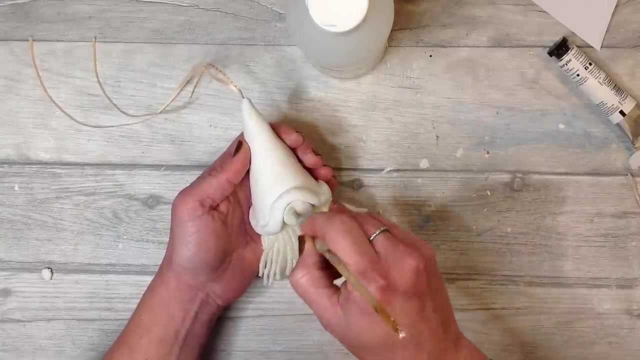 I'm going for the Nordic neutral look with these, but you can paint them however you wish in lots of bright colours, but I'm just taking a slight bit of flesh colour and painting the nose. You'll then need to add some sealant over the top of these and then they're ready to. 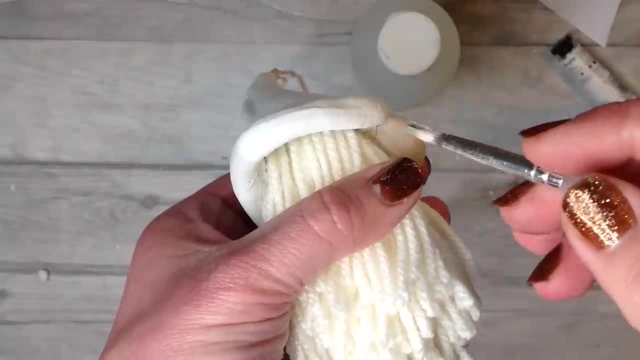 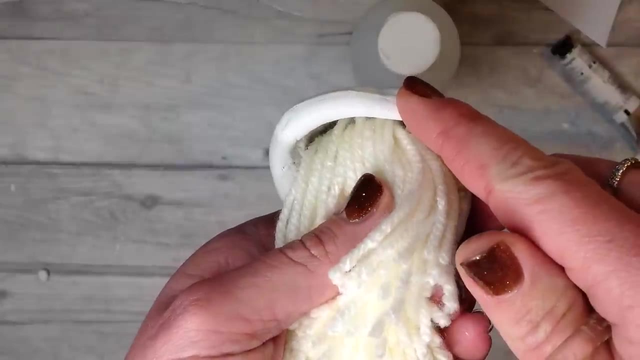 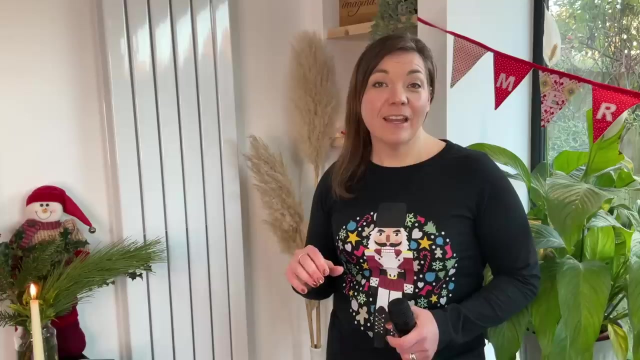 hang on your tree. When sealing the clay, make sure you do this in sections and let it dry in the sun. Then pull back the yarn so that this doesn't get stuck onto the hat. They're absolutely gorgeous. I really do love them. 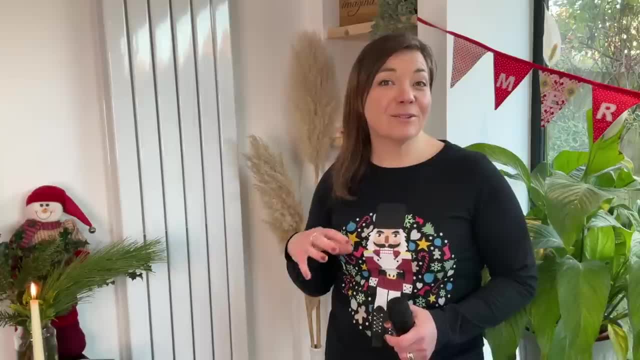 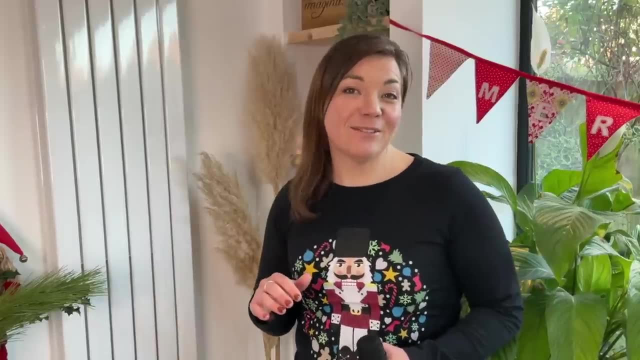 I really love the Scandinavian and Nordic feel to lots of Christmas decorations, so I'm keeping lots of them white and simple and neutrals, but you can add any splashes of colour you wish. For this next Christmas craft, I have some log discs. You could use discs of any colour. 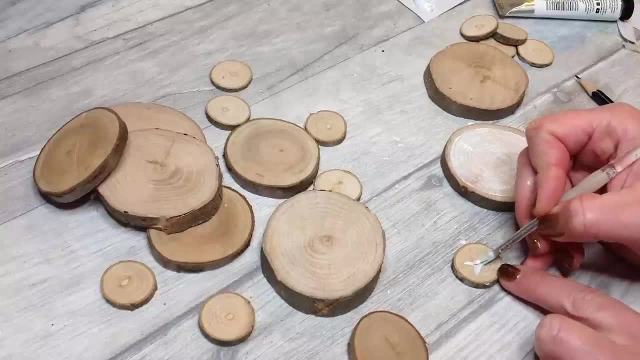 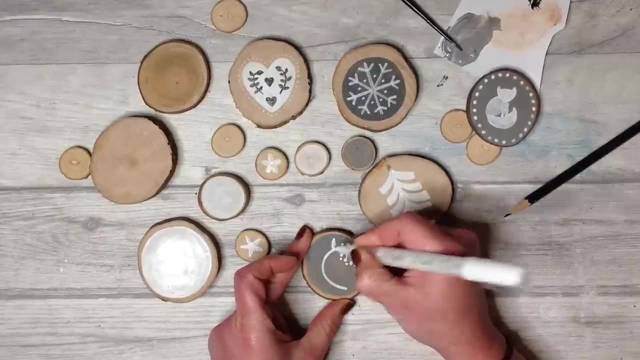 You could use discs of any colour. You could use discs of clay or even discs of card for this. Take some acrylic paint and just enjoy painting on any designs you wish. Again, I wanted to go for a bit of a Scandinavian feel, so I'm painting them some nice neutrals. 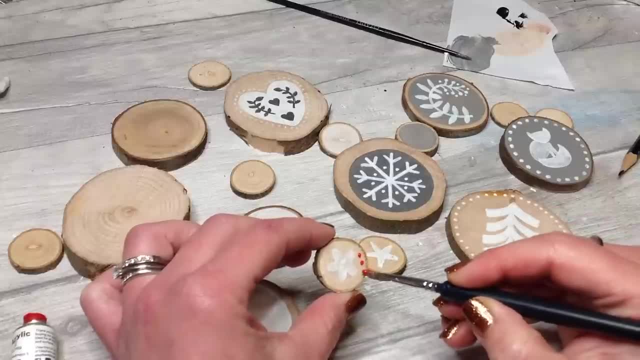 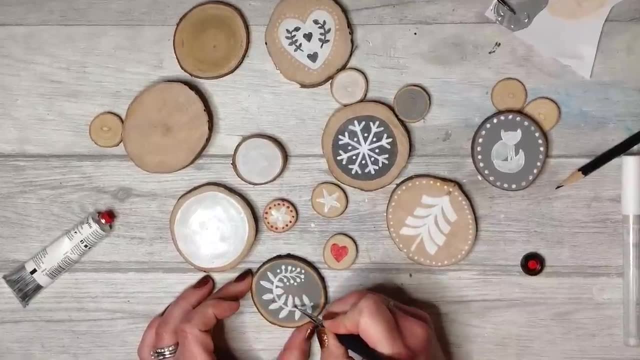 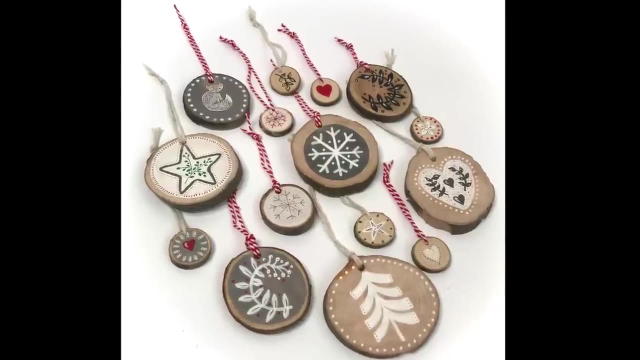 and just some little pops of red and green. This is a lovely, relaxing craft you can hopefully enjoy at Christmas. You can find some inspiration on places like Pinterest And hopefully get everyone involved. I drilled a hole in each one and added some cute ribbons. 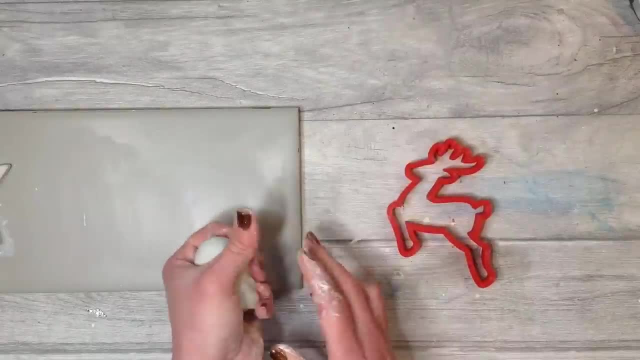 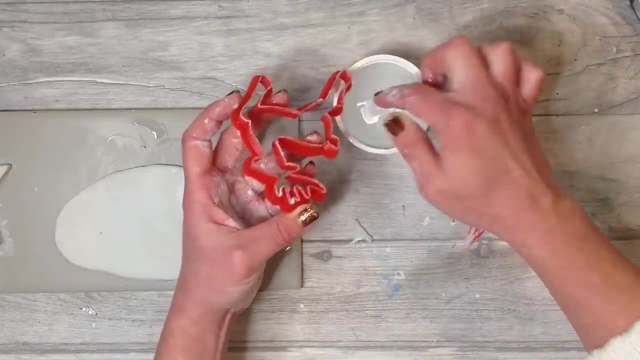 I'm back with my air dry clay And you really can get so many different cookie cutters and shapes to cut your clay out with. I cut this one on my 3D printer and I have another video where I show you how I do make. 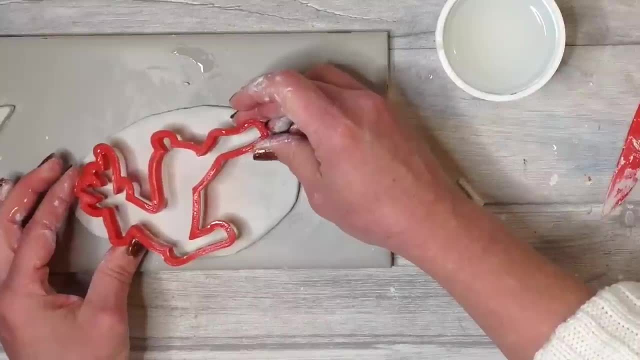 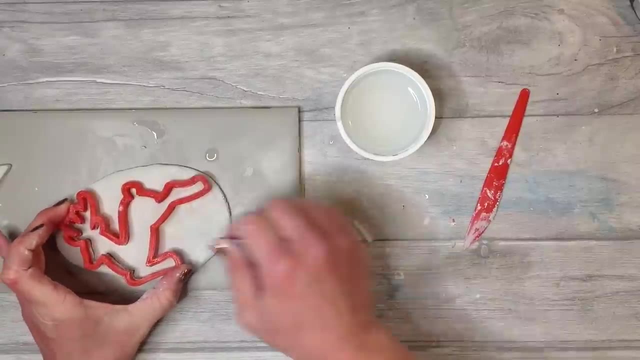 these on my 3D printer, if you are interested. Intricate cutters like this really can get stuck in the corner. I've added some cute ribbons here and there. So that's it clay. so my little tip, as you could see there, is to add a little bit of water all around the edges. 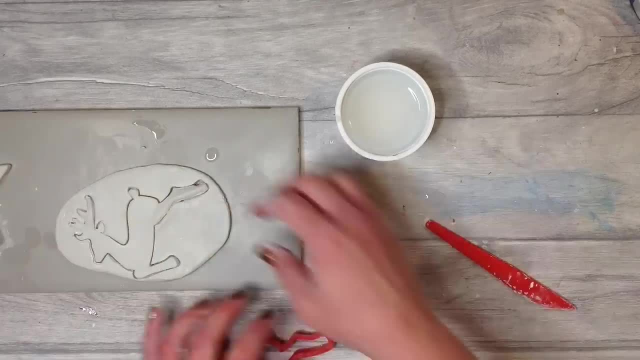 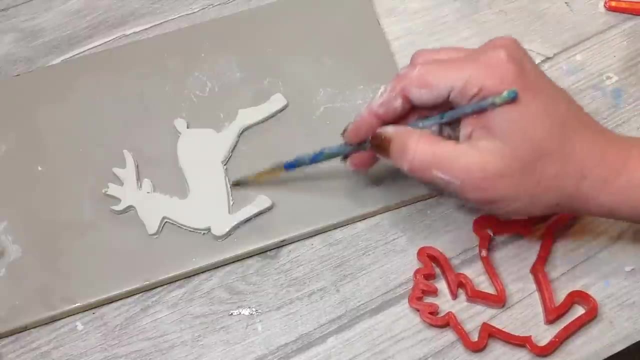 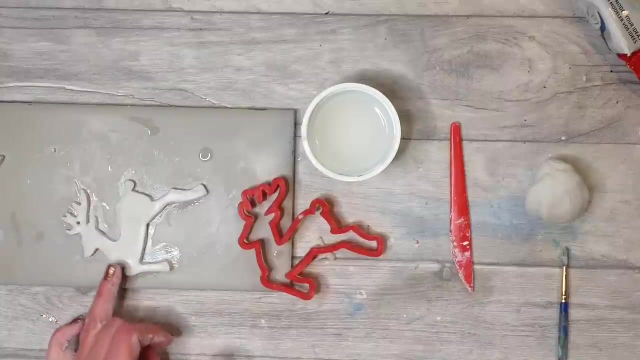 and then the cutter should slide off and prevent us from having to poke that clay like that too much. I always leave these delicate designs to dry on my tile, and that way we don't disturb them and they dry beautifully. Don't forget to add a hole in the top so that we can hang these on. 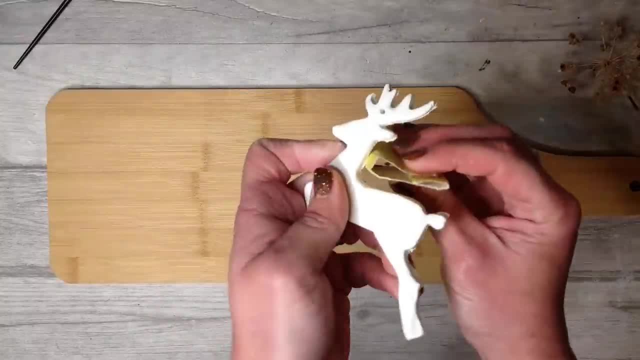 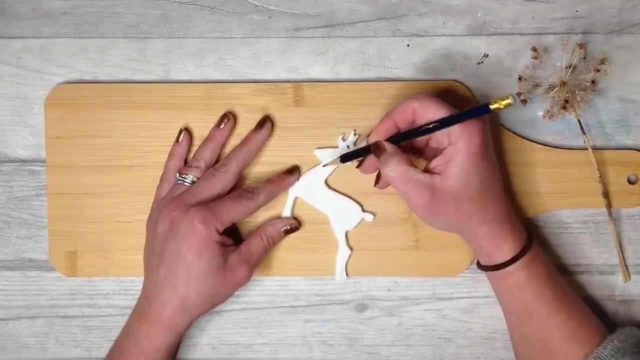 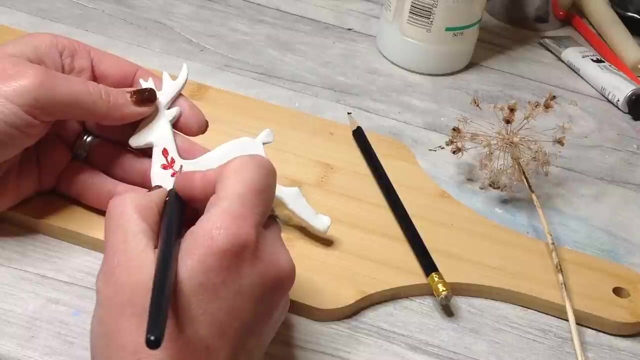 the tree. Once dry, I take the sandpaper to them and then I can paint them or add any designs and details I wish. Most often I like to keep them really simple, so I'm drawing on in pencil a little leaf design and a couple of hearts, and then with a very fine paintbrush I can paint these on with. 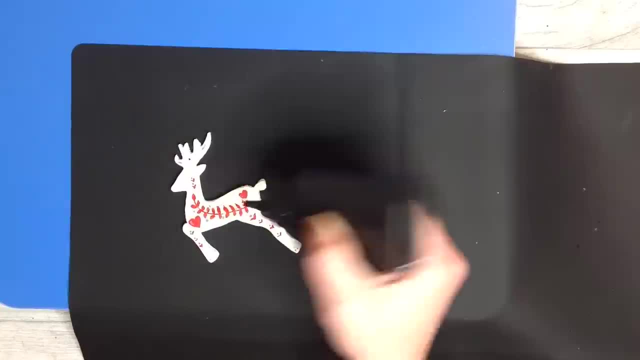 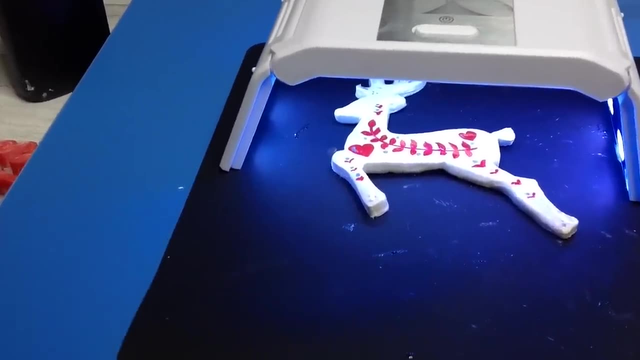 acrylic paints. To give these reindeers a really good shine, I'm using some UV resin. I'll link the products that I use in the description below. I'll link the products that I use in the description below. You really can make any shapes you wish and the resin just gives them that extra bit of. 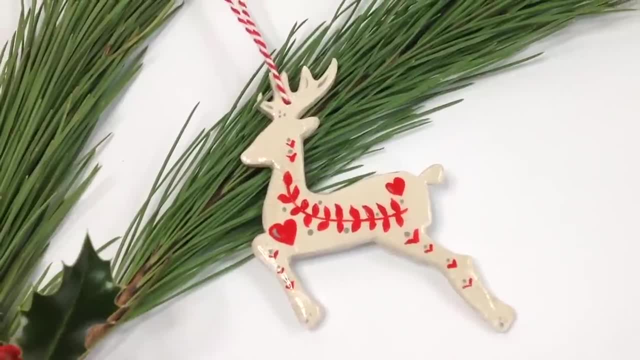 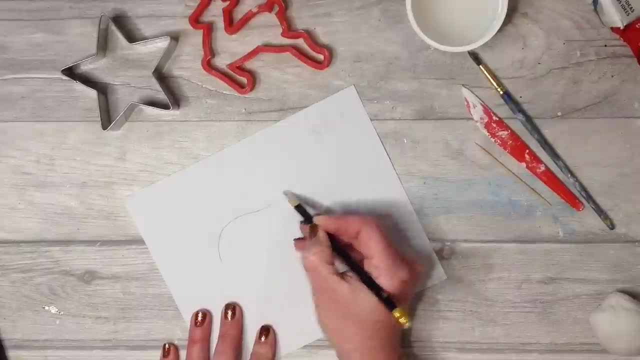 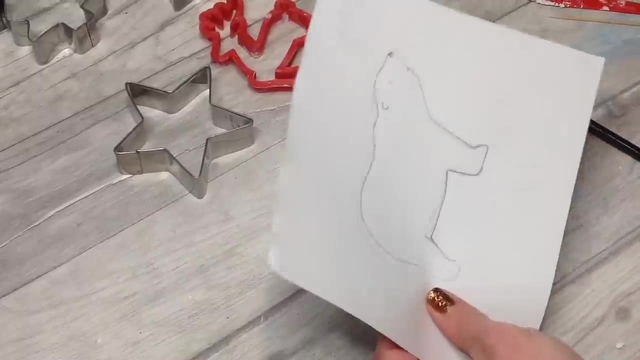 strength, and I think these look absolutely stunning. If you're thinking you don't have the cookie cutter that you'd like, then don't worry, there's always an alternative. I love to draw out a new design on paper. cut this out and use this as a template. You could print something off the 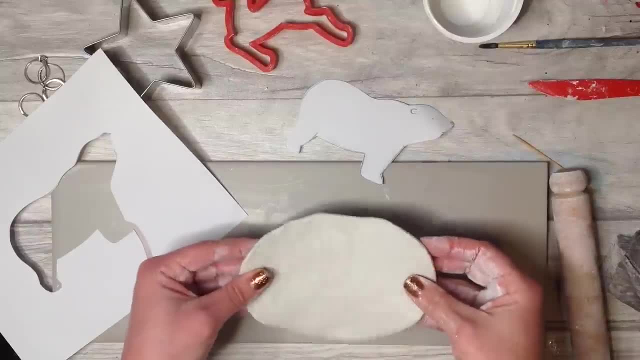 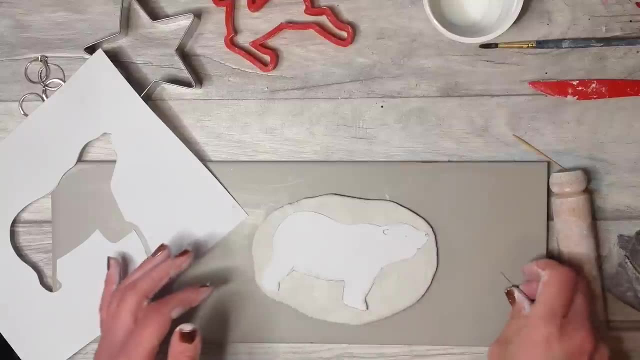 internet and cut this out and use it as a template. If you don't have a cookie cutter, you could cut this out in the same way. The beauty about air dry clay is you don't need lots of fancy equipment either. If you don't have a craft knife, then you can use something like a needle or a pin. 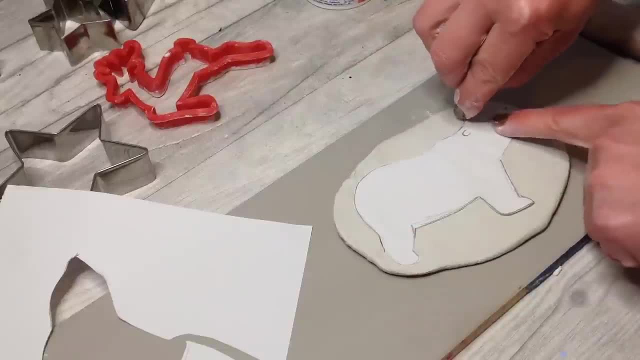 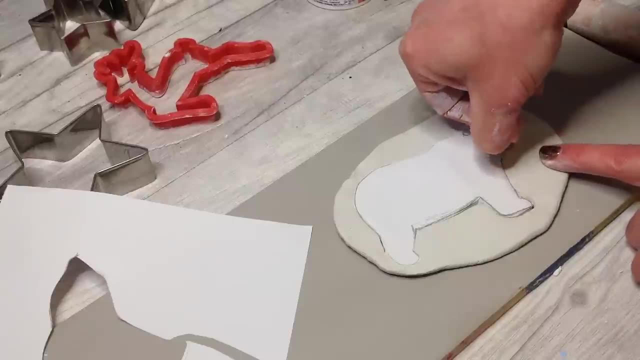 Place your paper template on top of the clay and then cut this out, running it all the way around the edge, pressing all the way down into the tile And just like that you have a really cute decoration With your finished design. you're ready to go. 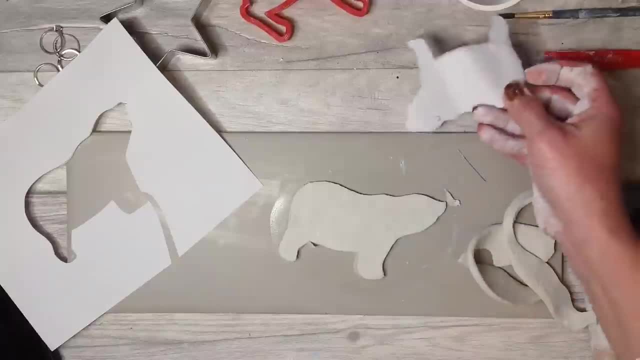 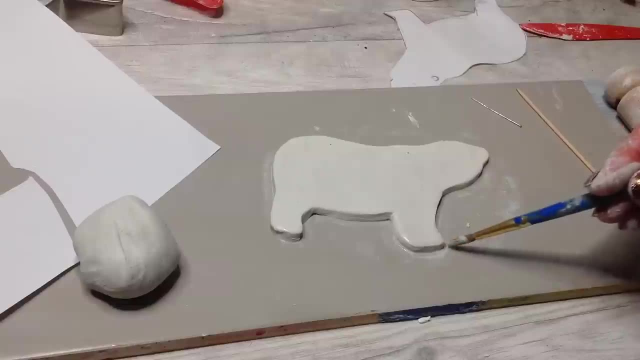 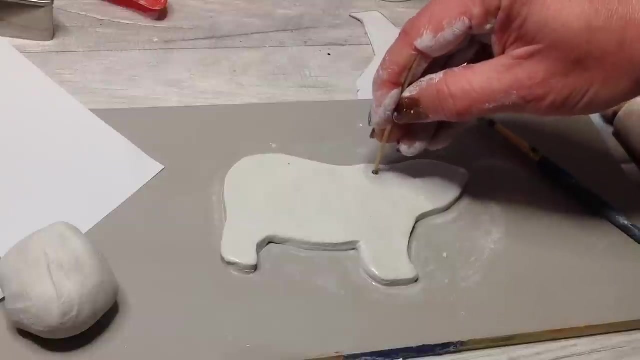 With a finger or a soft brush, neaten up the edges just with the tiniest bit of water. I'm so excited to see all these Christmassy things coming together With a cocktail stick or a straw. make two holes at the top. 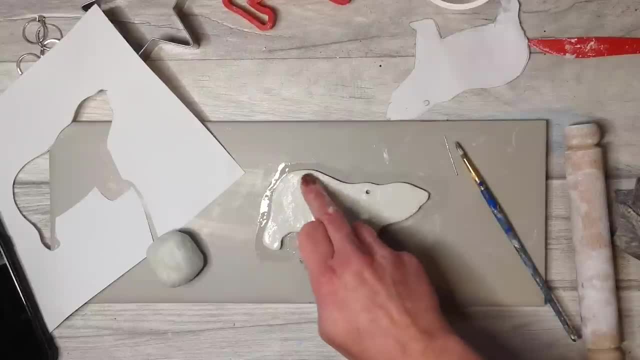 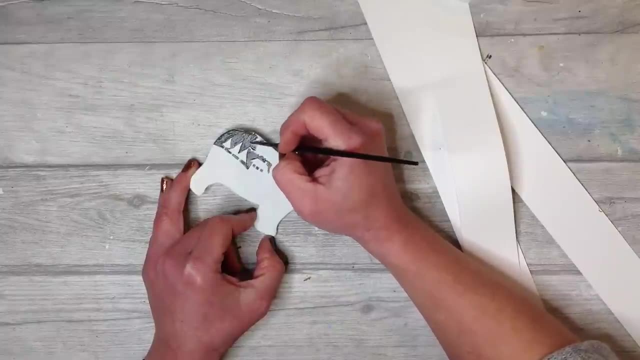 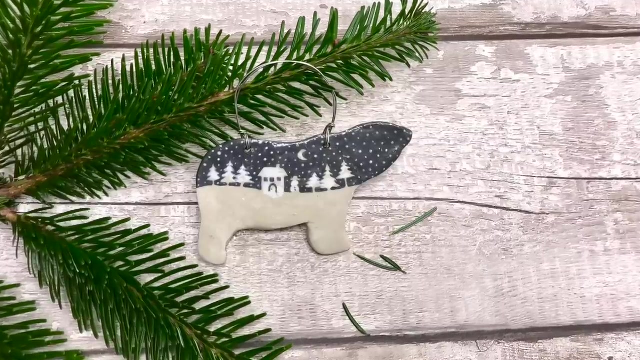 Two holes will just make it hang that little bit better for this kind of shape. Once the air dry, clay is fully dry, I take some acrylic paints and paint on it a cute little seam, Coating in resin and adding some wire. And here we have another one which turned out super cute. 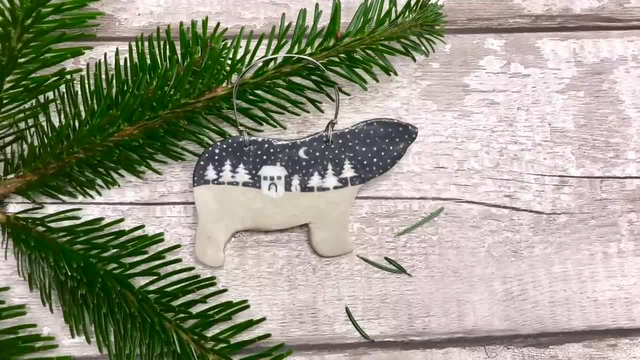 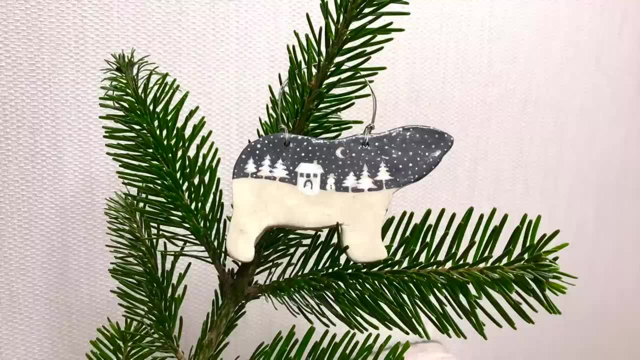 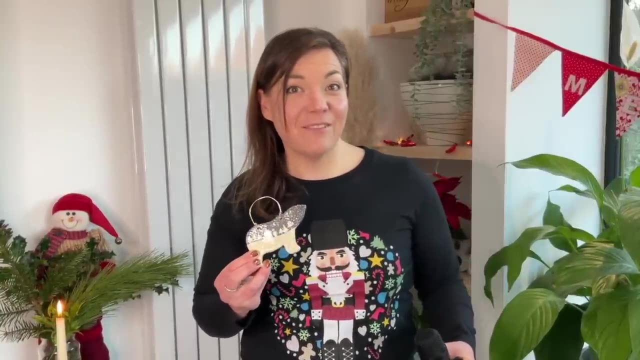 After painting in resin you can see the difference between the bare air dry clay and what is painted with white acrylic paint. If you want it really crisp white, make sure you paint it with white acrylic paint. Adding the wire to the top like this makes them look really expensive and really lovely and 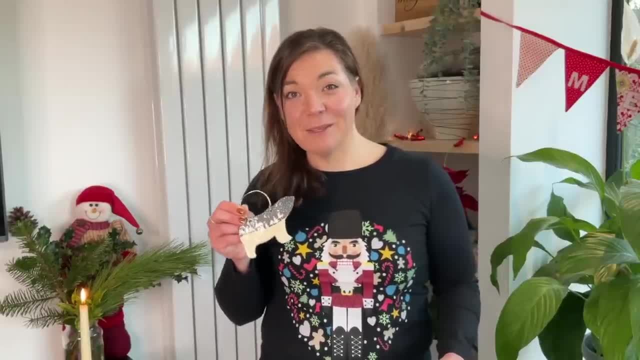 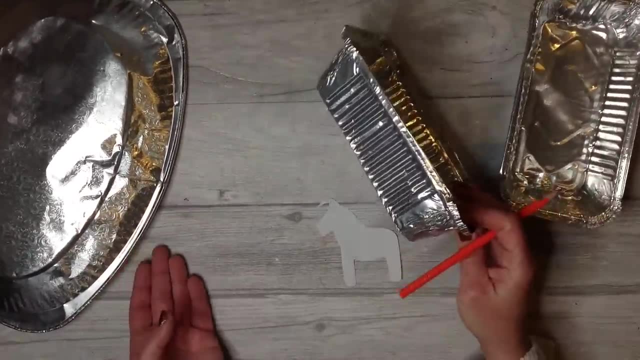 handmade. I really hope you give these a go. I think they're super easy to make and I'm sure you'll love them. I think they're super cute and I'll definitely be making some more. Tin foil trays are another really fantastic craft medium. 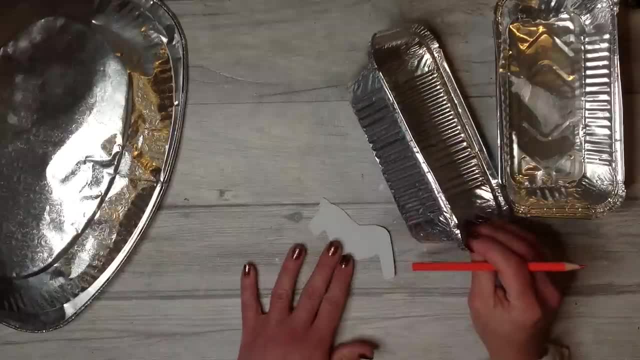 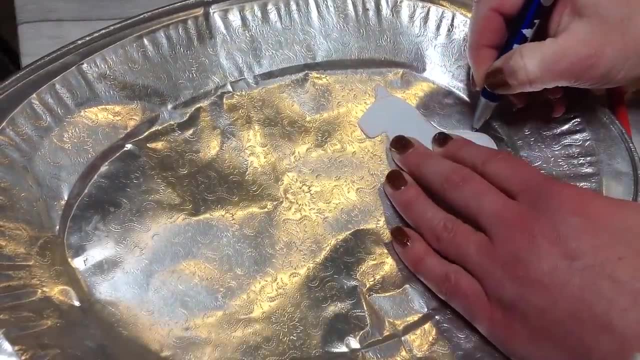 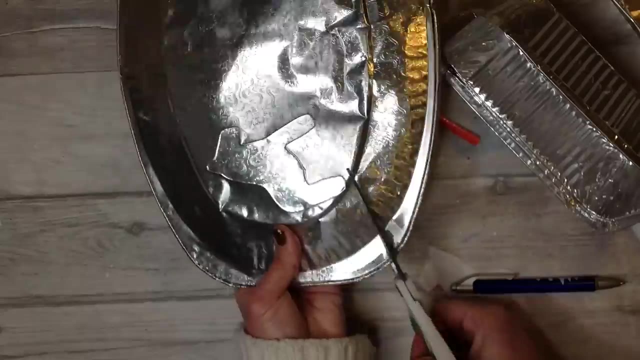 and let me show you how I make some Christmas decorations out of them. I've drawn and cut out a Scandinavian style horse and I'm going to trace this onto the tin foil Using a ballpoint pen. I've pressed into the tin. Then we need to cut all the way around the edge with a two millimeter allowance. 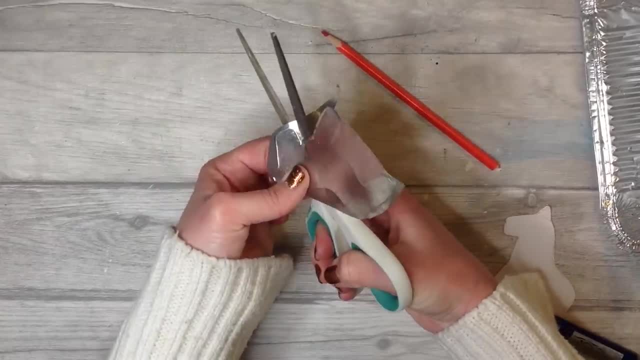 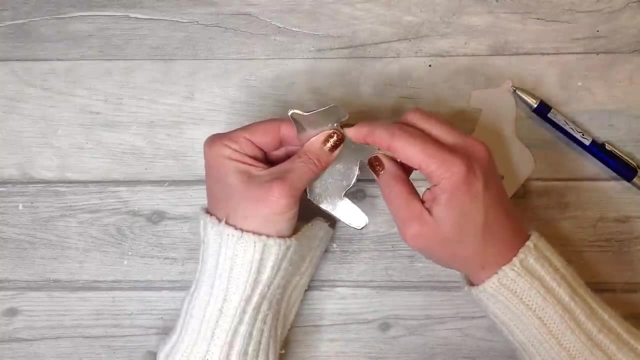 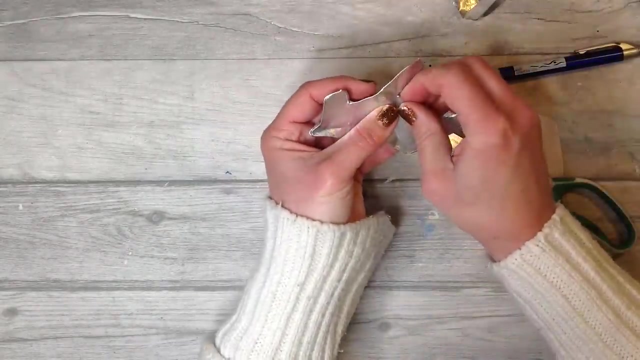 This project is definitely not a children's craft. The edges are very sharp so please do be extra careful. To try and help that sharp edge, I tuck over the extra two mils from all around the rim. Any tight corners you might just need to give a little snip. 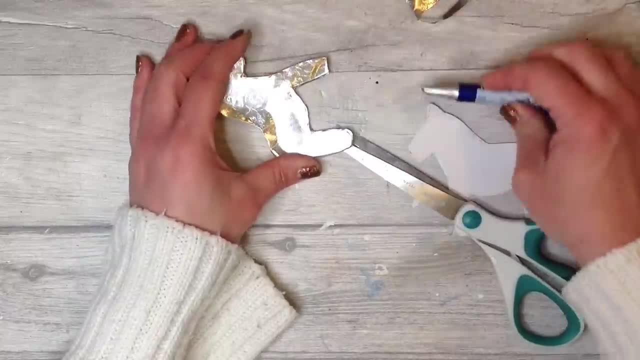 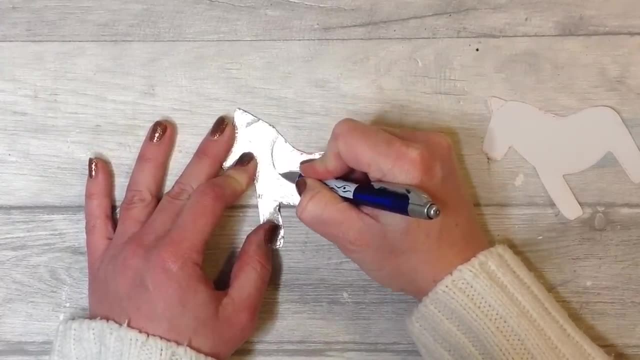 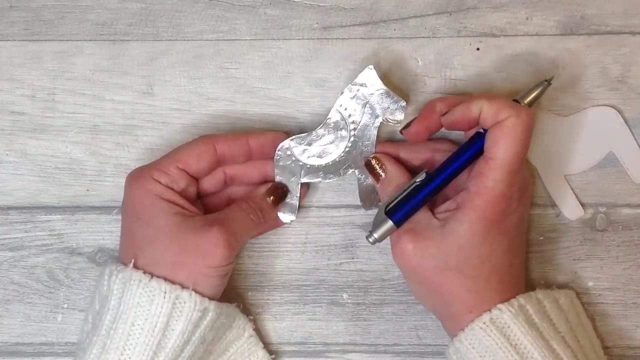 Press the edges down to make it lovely and neat. Turning the decoration onto the back, we can take our ballpoint pen again and add in some lovely details. This is another fun and very effective craft and I certainly enjoy making these at Christmas time. The shine on these is beautiful and I really love that recycled element. 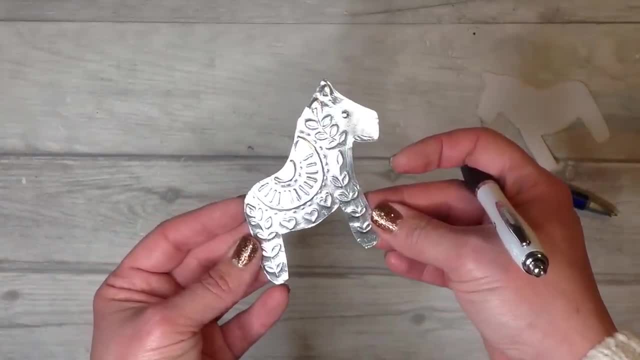 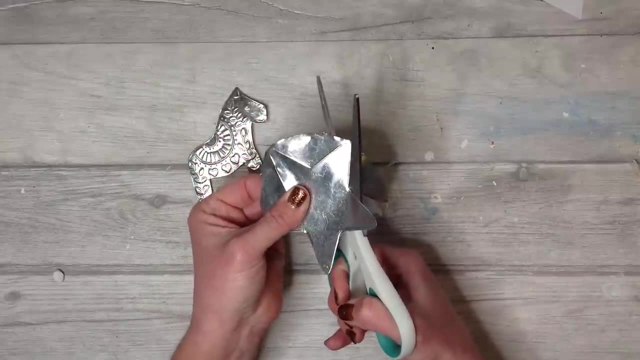 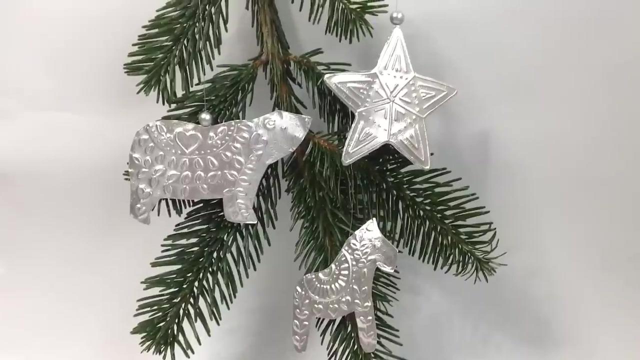 So next time you get an item of food in a tin foil tray, why not wash it and recycle it this way: With a pin or a needle, make a hole and add some thread. If you find the turning of the edges a little bit tricky, you can cut on your first line. 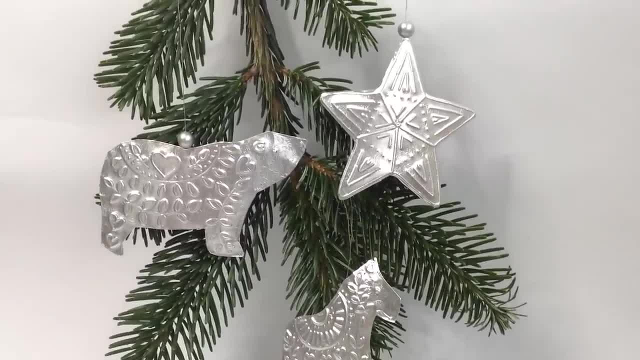 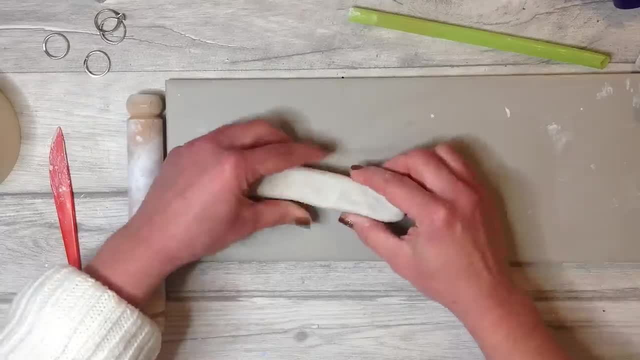 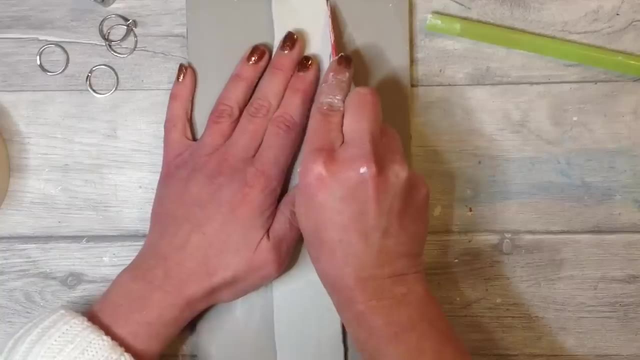 And then outline with a nice edge- Just be careful that they're not too sharp- and do some nice soft edges. To make this next one, I have a thick coil of air dry clay that I'm rolling nice and long and thin By eye or with a ruler, cut a nice shape out like this: 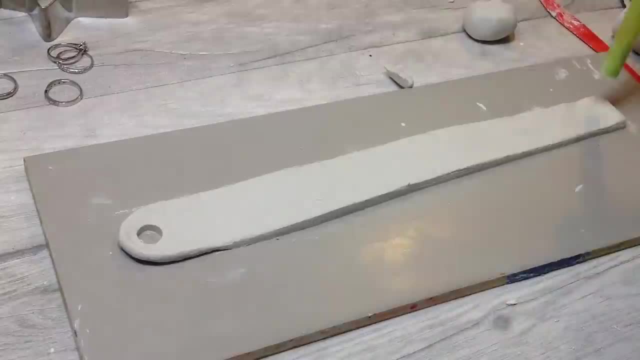 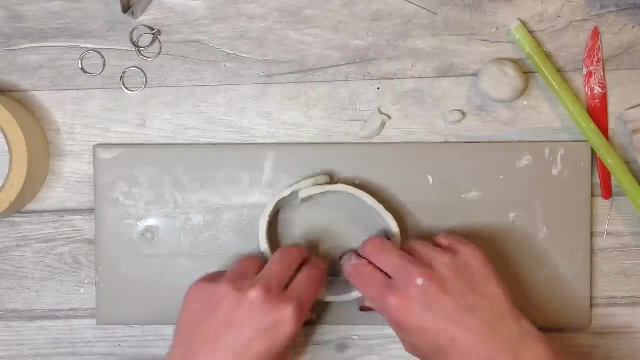 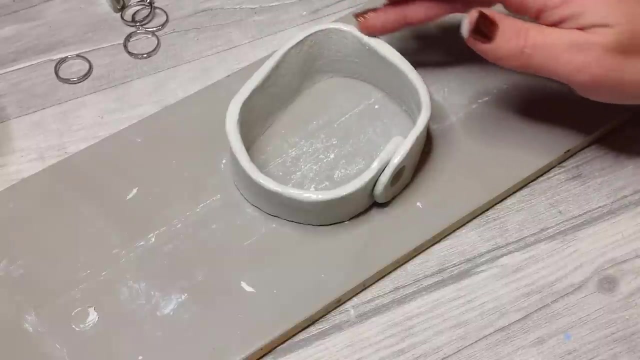 Well, this project does work. lovely and rustic too. With my thick straw, I'm cutting out A hole out of each end. Bring the two ends together and match up those holes. This is going to hold some dried flowers, so I make it flat on the base. 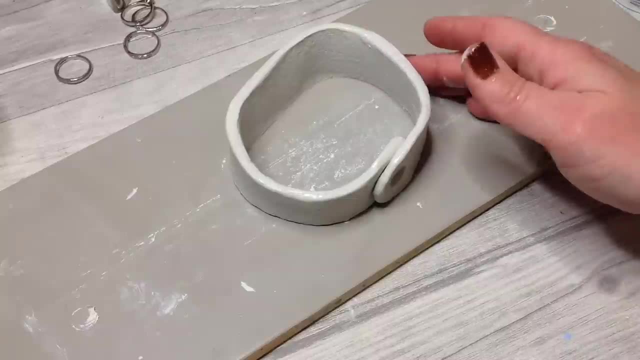 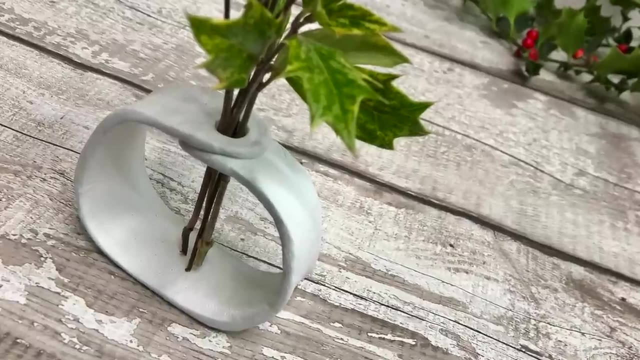 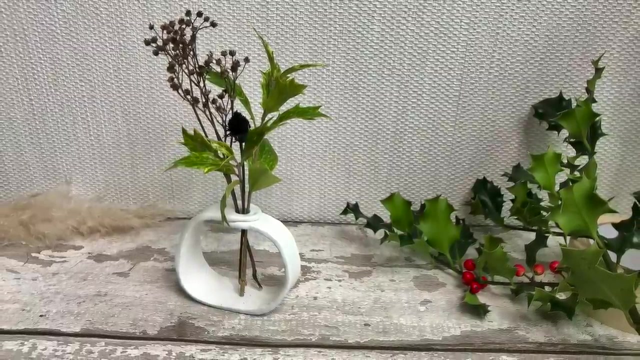 The holes will be the top Once again. leave this air dry. clay to dry naturally, nice and slowly. I really love simple and effective pieces like this and it really looks lovely with some Christmas foliage. I have a paper craft for an alternative Christmas decoration for you. 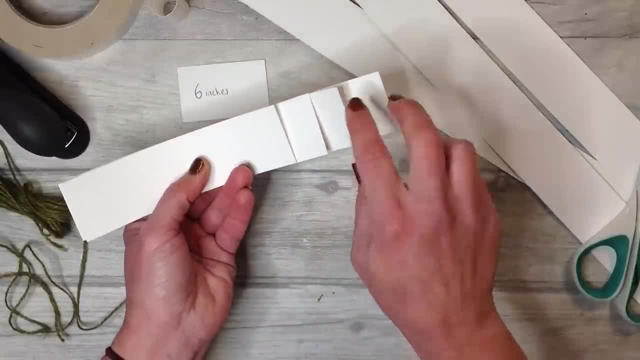 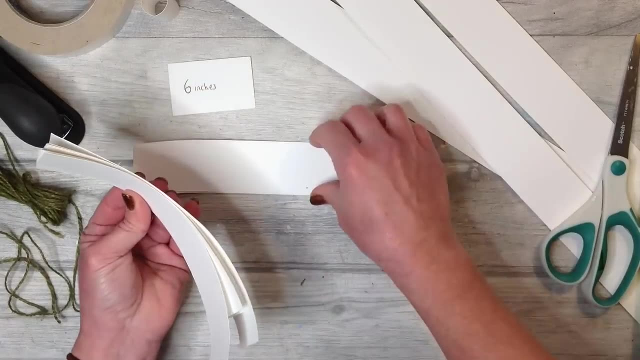 I'm starting with some strips of thin card. The first two pieces are six inches, and then each two are going up at about an inch bigger each time. Start with the small ones in the center and then go either side with each next size, as I have here. 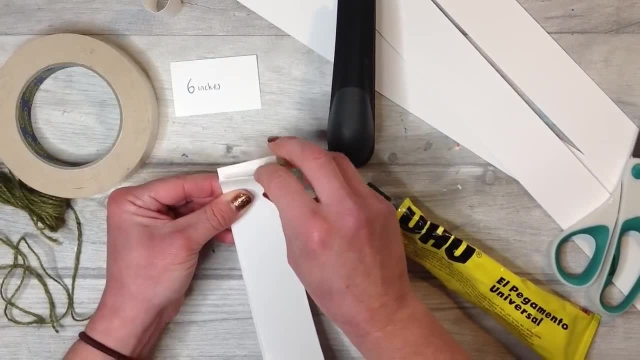 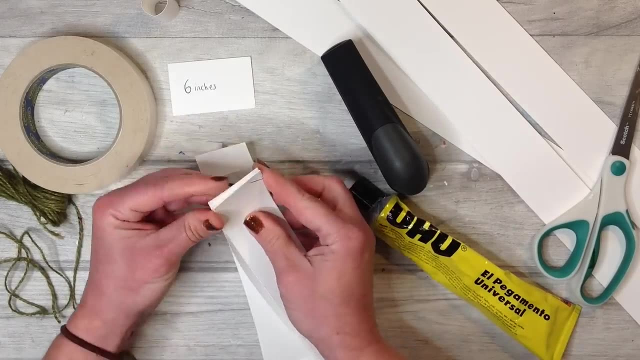 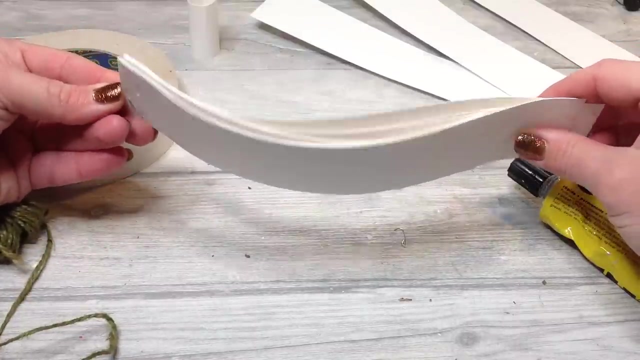 Glue tape or staple one end together. I'm stapling them and I just do A few together at a time. Hot glue is a good option as well. Once the first end is nice and secure, we can take the two center pieces. 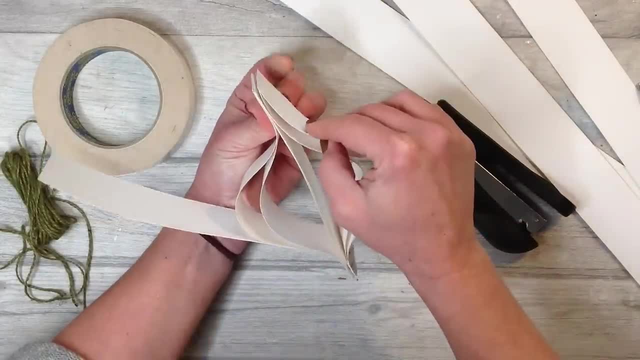 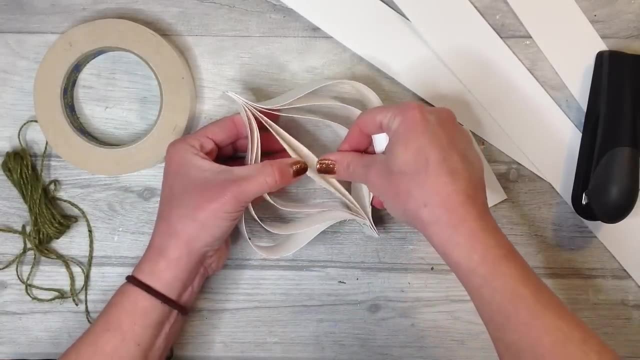 and then join the rest of them together like this, so that they all meet up on the end, Glue or attach together as before. and then I take a small bit of card and make this into a coil and I'll attach this into the middle. 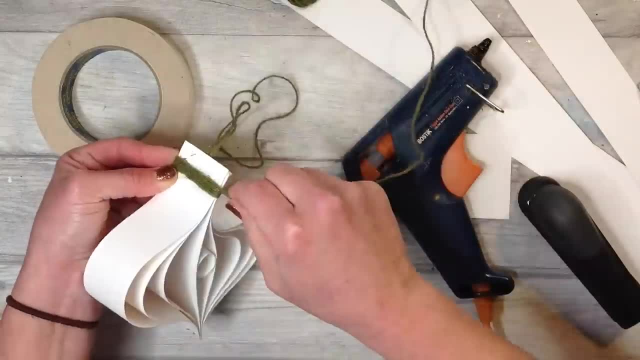 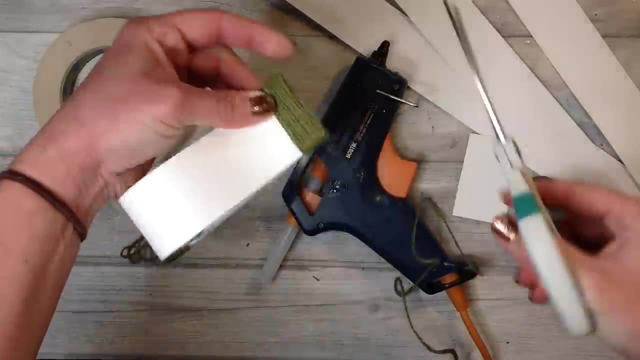 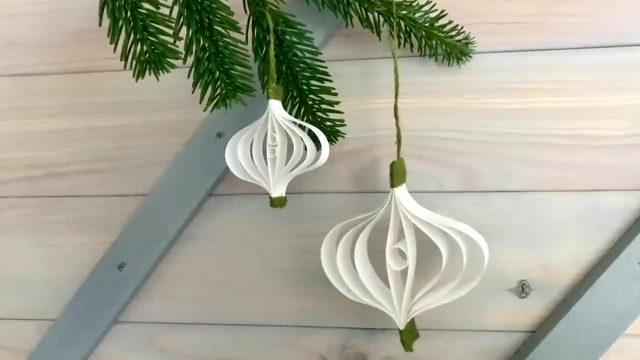 Add a piece of string so that this can hang up, and then, with the rest of the string, I'm adding some hot glue and making it into a nice neat pattern. Repeat this on the base and why not make them in lots of different sizes. Another easy and creative decoration that can be from your recycling. 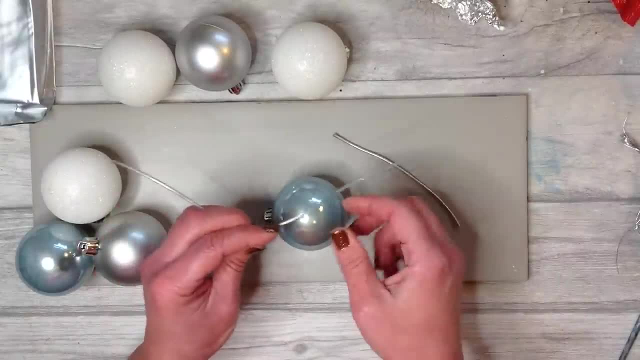 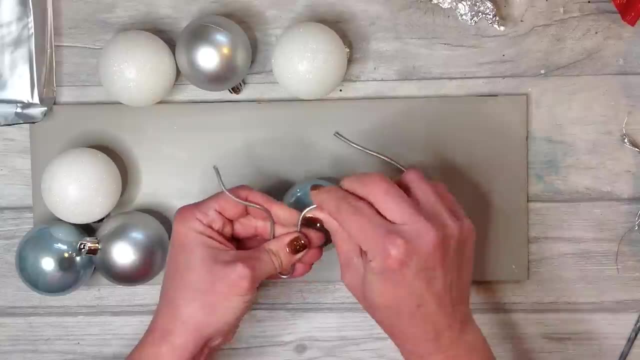 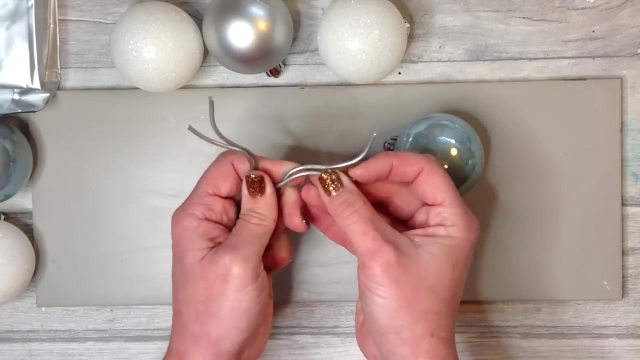 If you think you've enjoyed these crafts so far, I think this one really does have to be my favorite. I'm transforming these ordinary baubles into something even more beautiful, First of all taking some craft wire and bending it like this. We'll then need some tin foil and a glue gun, and this will also then be using air dry clay. 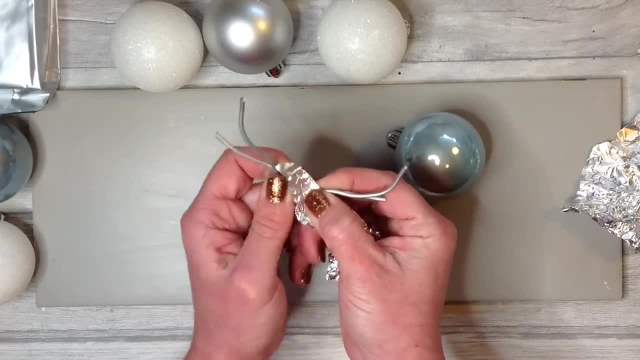 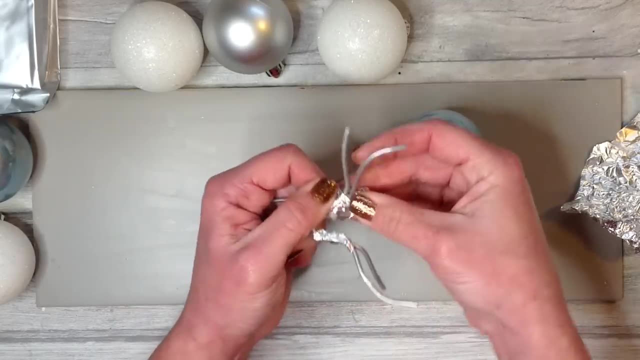 With the wire and tin foil I'm creating a stag's head shape or a reindeer shape. The first bit here can be a little fiddly, but once you get going it does get easier. Use a little hot glue if you are struggling to hold this in place. 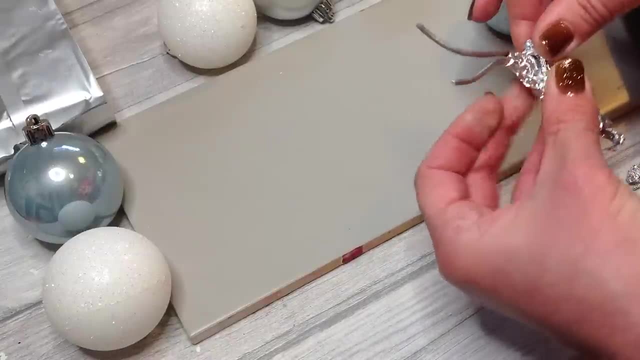 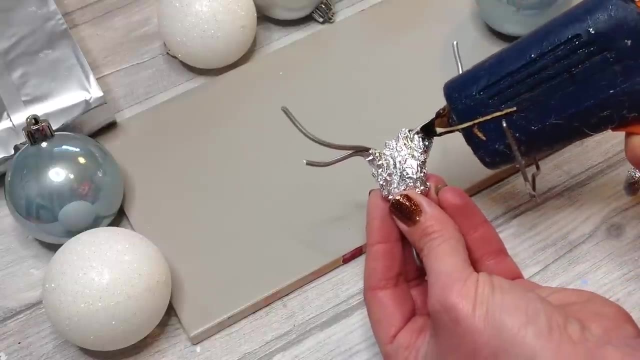 I'm hoping that these videos will give you the inspiration to pick up some craft materials and have a go yourself. My kids love to craft and create with me as well, and I always say it doesn't always matter the finished result, just enjoy the process and have. 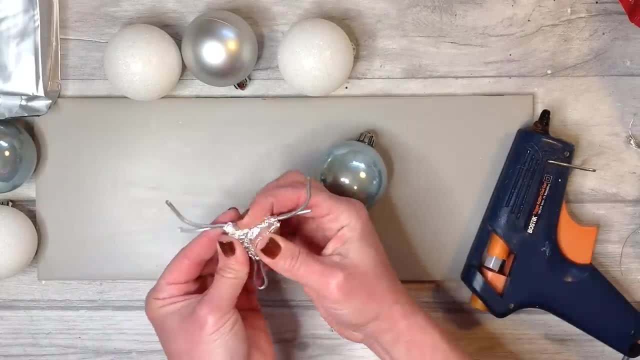 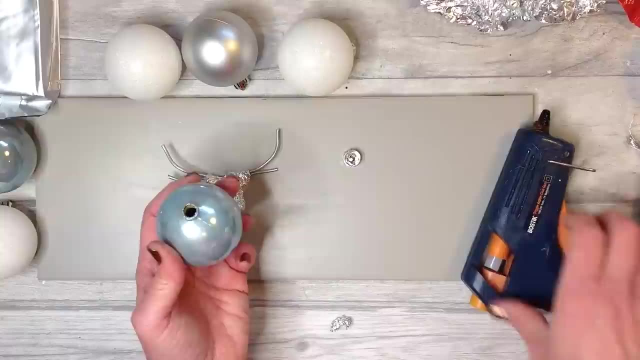 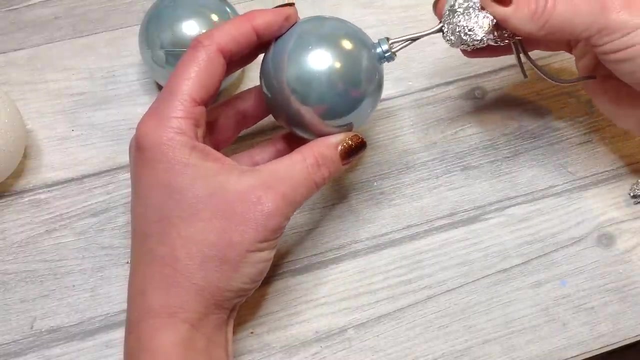 fun with your craft. I'm building up the shape with the tin foil and making it nice and secure. So I take some hot glue, insert it into here and then add in the wire and this gives it some really good stability. I continue to build up the profile of the stag with some more tin foil. 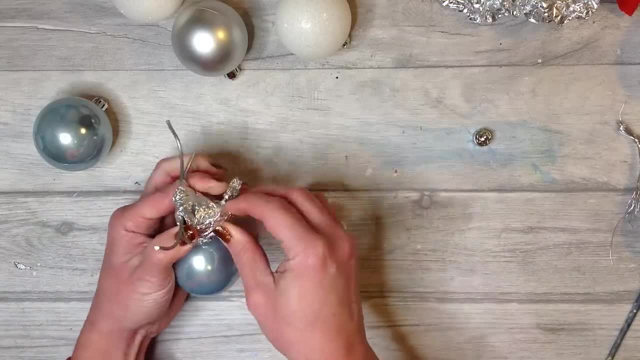 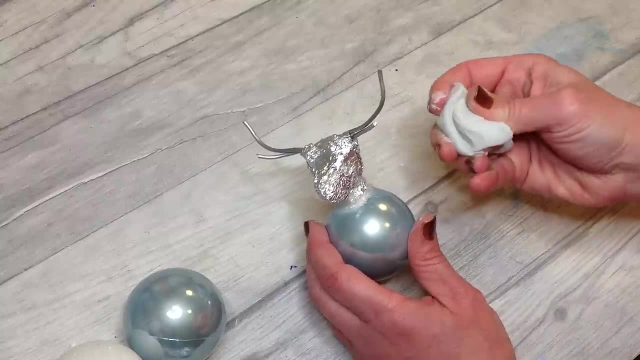 and add a little bit of hot glue to hold everything into place. I've given the air-dry clay a good knead to soften it up and it's now ready to use. You can roll some clay into the tin foil if you like. 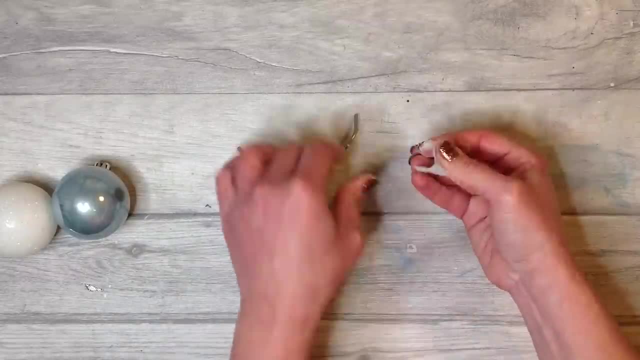 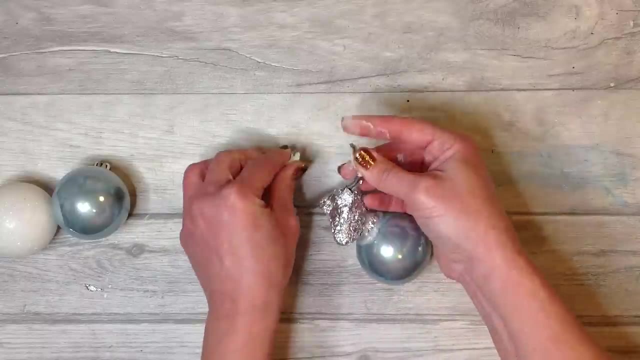 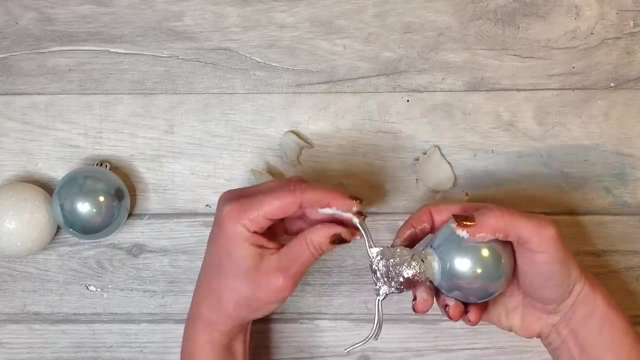 I like to play out thinly, if you wish, with a rolling pin, but I like to pinch small bits between my fingers for this small piece and pinch it and mould it onto my structure. The idea is we want to cover the whole of the head and the antlers in the air-dry clay. 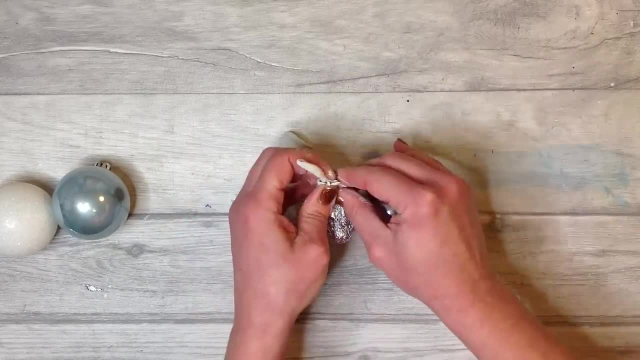 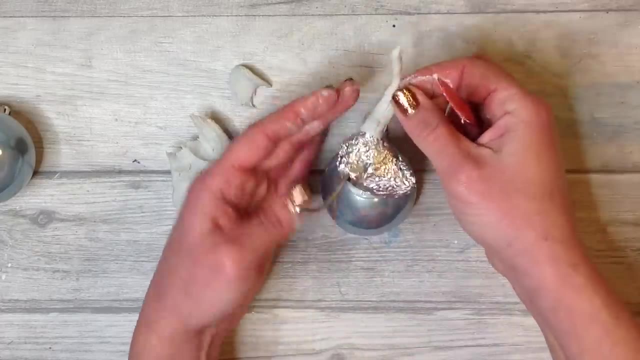 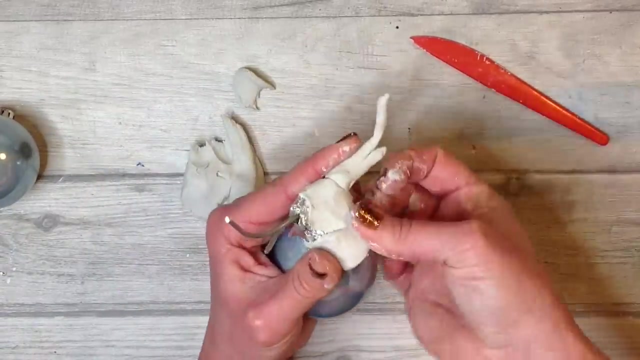 completing a small section at a time. As the clay is nice and soft, it moulds together really quite easily. This is one of these pieces that you really can't believe it's finished. it was made from air-dry clay. Over here on my channel I have lots of different craft projects. 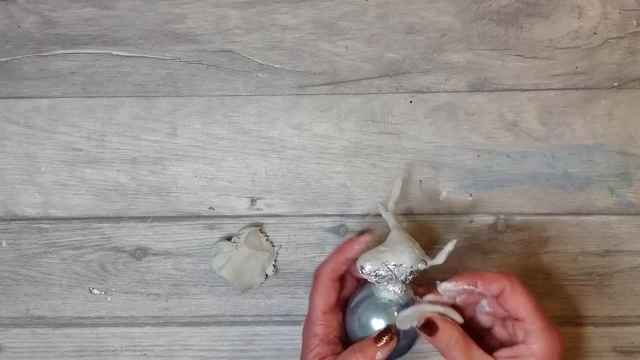 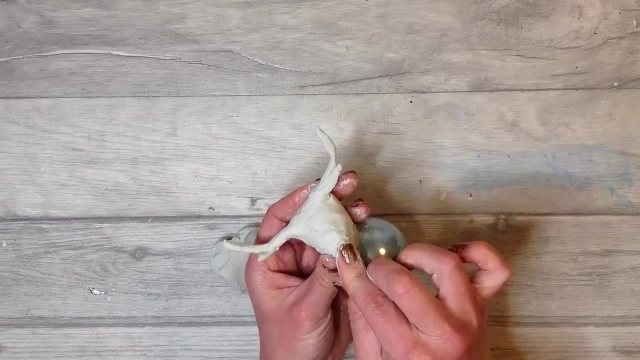 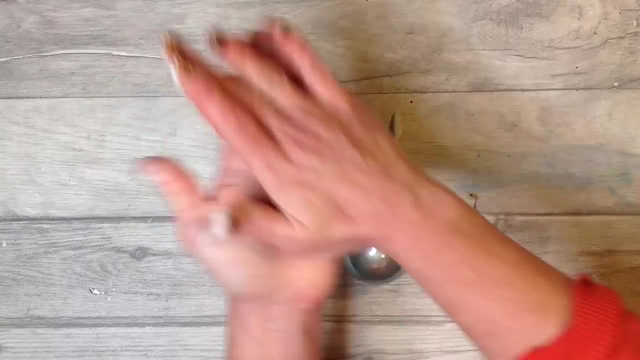 but an awful lot of air-dry clay projects, so please do come and look at some more. Don't forget to hit the subscribe button and the notification bell as well, so that you don't miss any of my craft videos. There are ways to support me as well, so I'll put those in the description below. 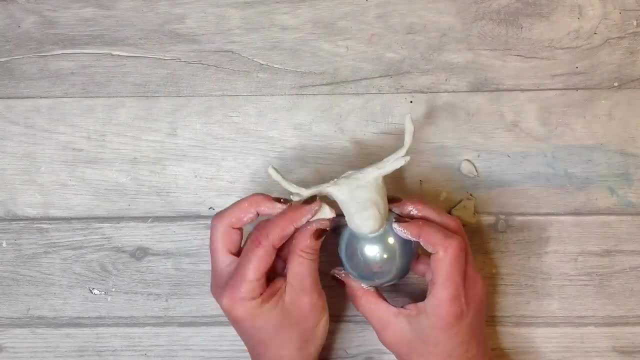 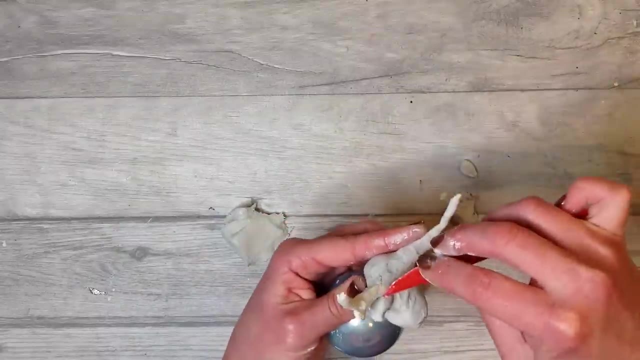 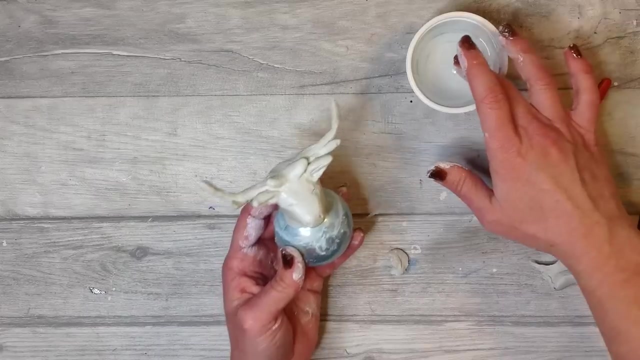 I want to give my stag some ears so I can add these details on quite easily Just shaping the ear shape and then blending this in the correct spot With a basic tool or a pencil you can add in some details. I'm adding in some extra details to the antlers and then some eyes, the nose and the mouth. 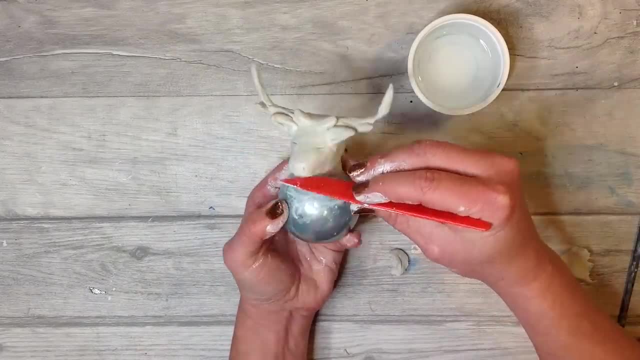 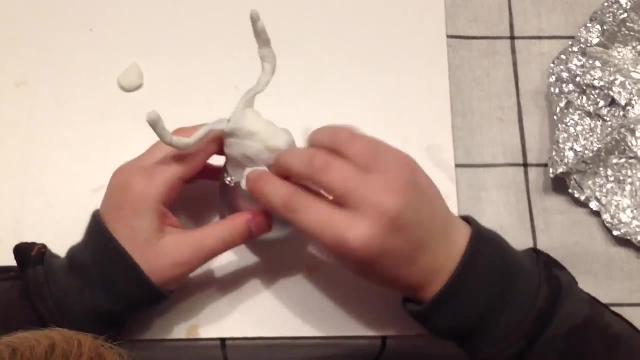 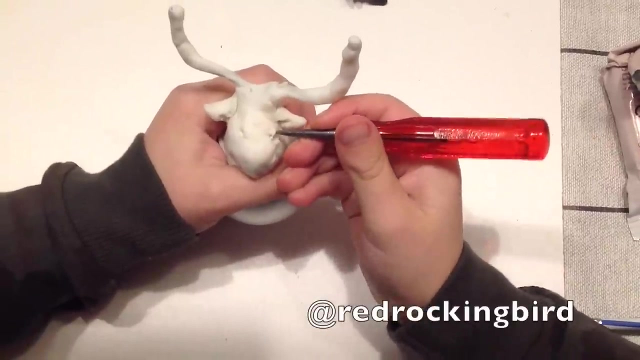 Taking a small amount of water and smoothing everything out. My youngest son is here next to me making his own, and I couldn't be prouder. I think his looks like a moose and I really love it. Don't forget, you can follow us over on Instagram as well. 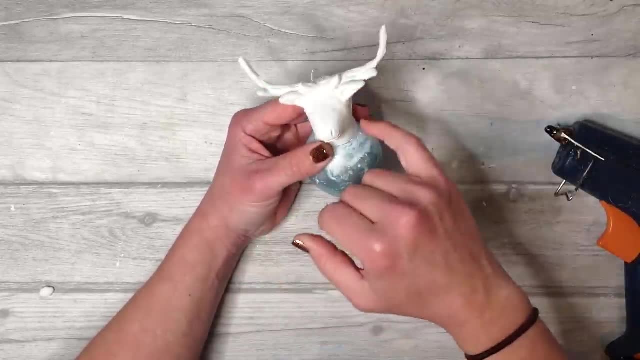 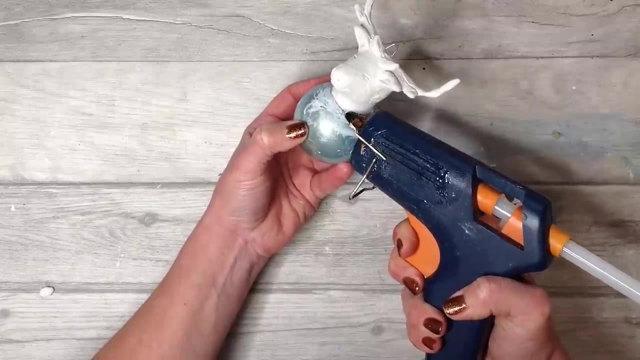 They're now fully dry, a few tiny hairline cracks have appeared. You can either fix these or you can leave them to add to the effect. To add a little bit more detail. I have a hot glue gun and I'm adding some detail onto the bauble.